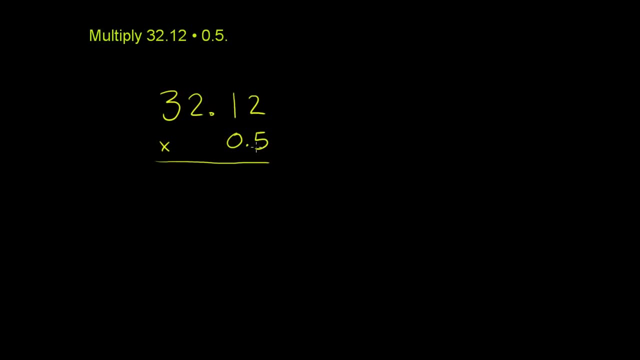 But you can almost pretend that this is 3,212 times 5.. And then we'll worry about the decimals in a second. So let's get started. So if we were just multiplying 5 times 3,212, we would say: 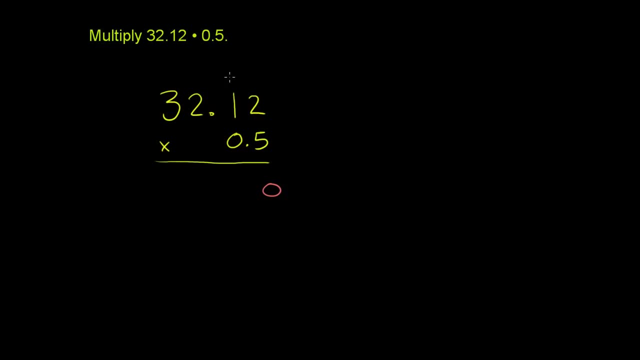 well, 5 times 5. 2 is 10.. Regroup the 1. 5 times 1 is 5. Plus 1. Plus 1 is 6.. 5 times 2 is 10.. 5 times 2 is 10.. 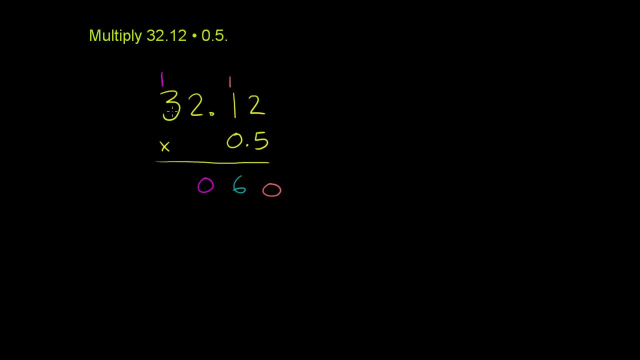 Regroup the 1.. And then finally you have 5 times 3 is 15.. Plus 1 is 16.. And then we don't have any other places. This 0 really isn't. If we were just viewing this as 0,, 5,, we wouldn't multiply 0. 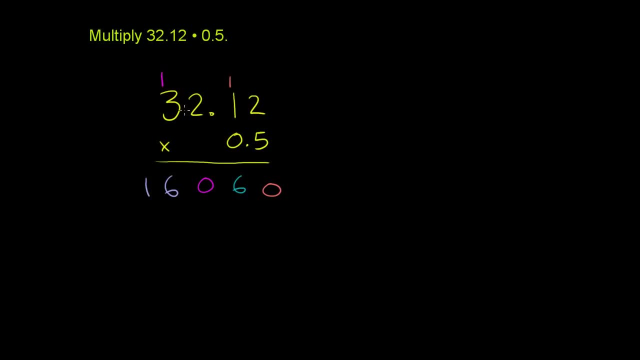 times this whole thing, We'd just get 0 anyway. So just 5 times 3,212 gives us this number. But now we want to care about the decimals. We just have to count the total number of spaces or places we have behind the decimal points in the two numbers we're. 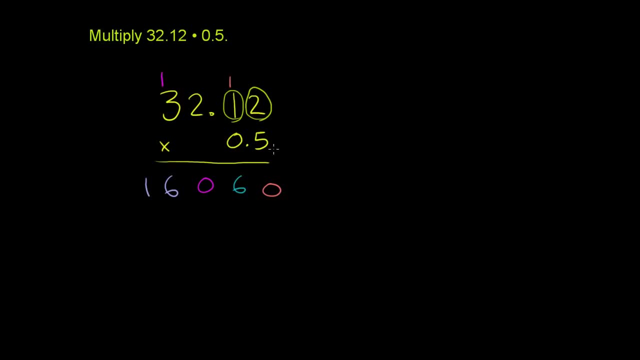 multiplying. So we have 1,, 2,, 3 spaces or 3 numbers to the right of the decimals in the two numbers that we're multiplying. So we need that many numbers to the right of the decimal in our answer. So we go 1,, 2,, 3, put the decimal right over there. 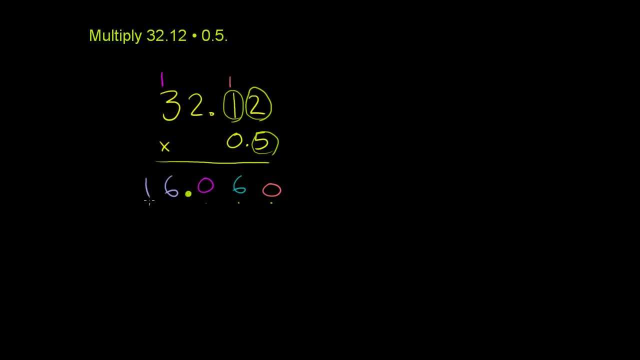 So 32.12 times 0.5 is 16.060.. And this trailing 0 right here we can ignore because it's really not adding any information there. So we could just write this as 16.06.. Now the last thing you want to do is just kind of make sure. 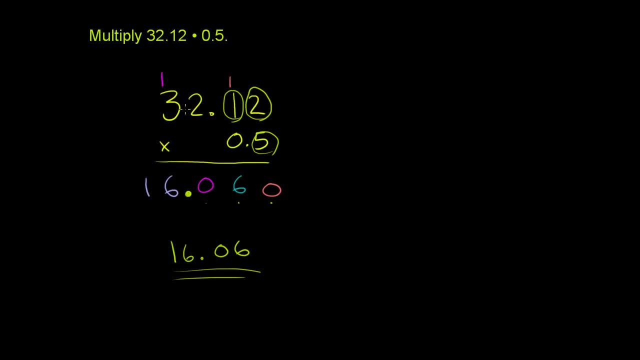 that this makes sense. You have a number that's almost 32.. And we're multiplying it by 0.5.. Remember, 0.5 is the same thing as 5 over 10, which is the same thing as 1.5.. 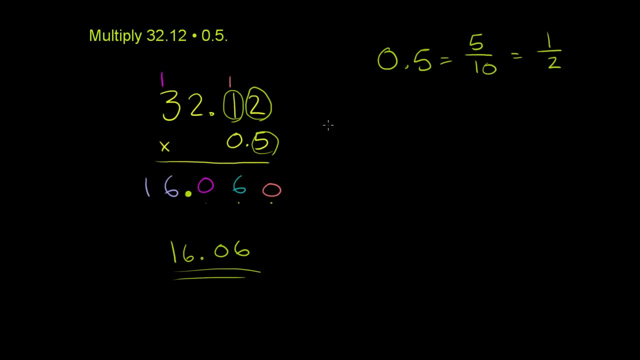 So we're really multiplying 32.12 times 1.5.. We're trying to figure out what 1.5 of 32.12 is, And half of 32 is 16, and then half of 0.12 is 0.06.. So this makes complete sense.